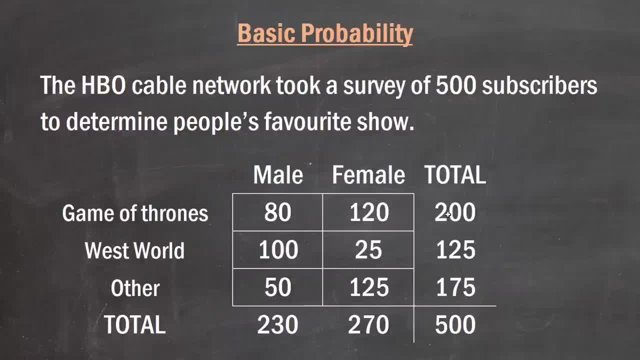 row where we just sum up the total number of people that thought Game of Thrones was their favorite show, and that's 200.. The total number of people that thought Westworld was their favorite show, and that's 125.. And we can also total up the males and females: it's 230 males and 270 females. But this 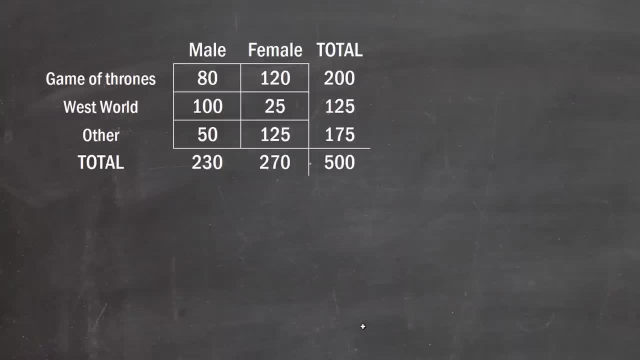 is not quite a probability distribution just yet. so let's see how we get there. Here's that distribution again. and if we divide everything by 500, which is the total number of observations, we get something which is called a probability distribution. So where before we had a 120 females who preferred Game of 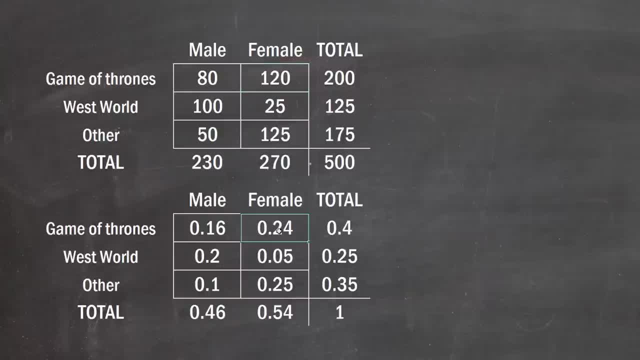 Thrones. we now have 0.24 in that cell, because that tells us that 0.24 is the number of people who preferred Game of Thrones, and so there's a or 24% of the distribution is defined by that joint event. So that's why we call that a joint probability. 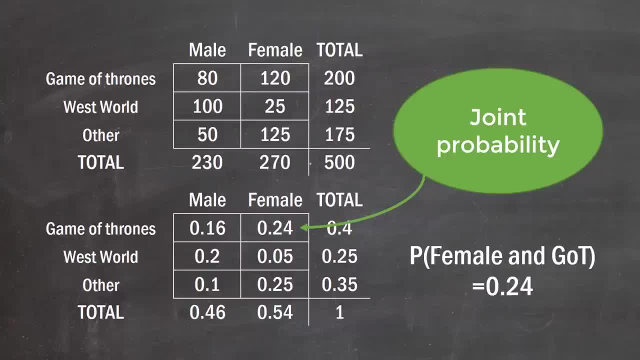 So that 0.24 is called a joint probability And the way we can write that is to say, the probability of female, the event where the person is female and the event where the person likes Game of Thrones is 0.24.. Now you might see it written with the word and in between: 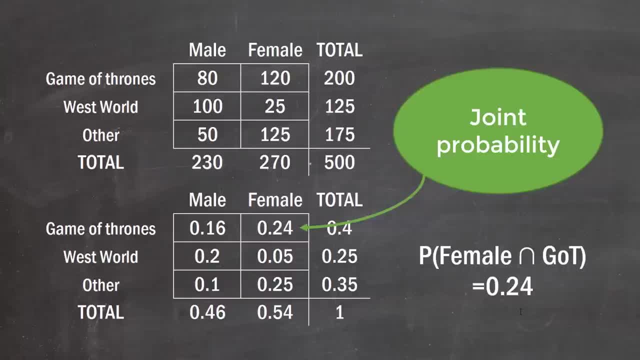 or else you might see it with this sort of upside down U which we're gonna call intersection- So that's just a fancy statistical term to say the intersection of female and Game of Thrones, which is of course that joint probability. Now collectively, those six cells here, 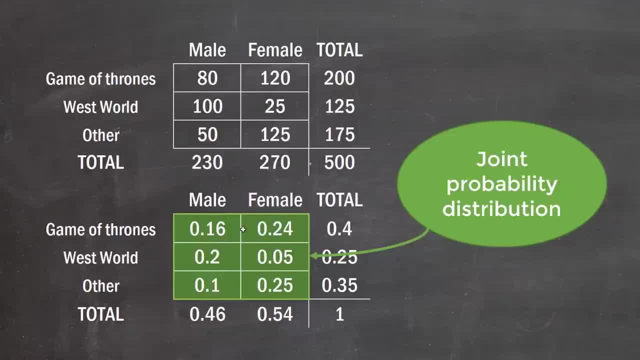 form what's called the joint probability distribution. So all of these six cells are gonna add up to one because, if you think about it, everyone in this distribution has to be in one of these cells. You have to either be male or female. 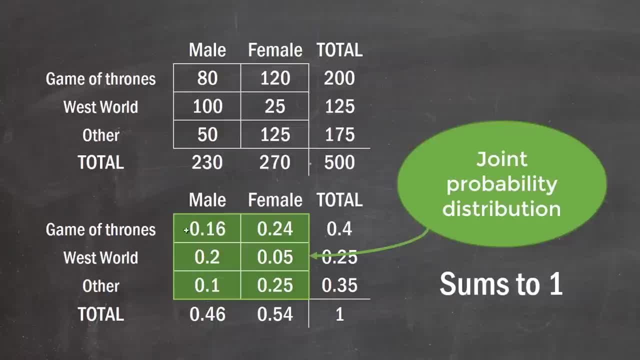 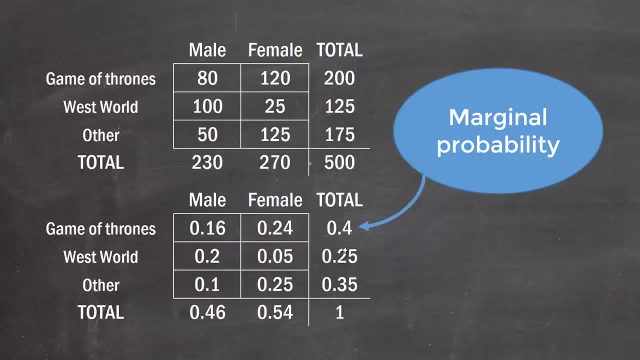 and you have to have selected one of these options. So it's no surprise that this should sum up to one. Now we can also go and calculate what's called the marginal probability- called as such because it's in the margins. Another term for this is the simple probability. 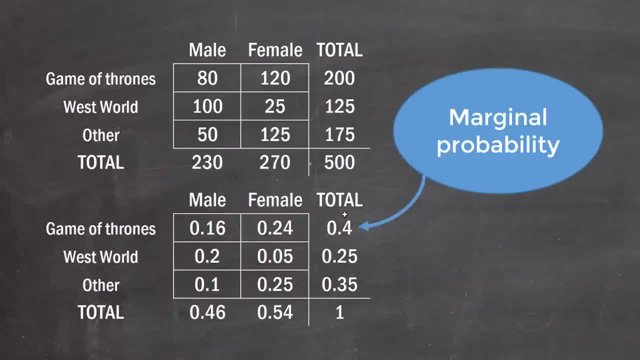 So just be aware of that if you see the phrase simple probability. but here this 0.4 refers to the raw probability of someone liking Game of Thrones, And I'm sure you can tell. it's just the sum of both the male and female joint probabilities. 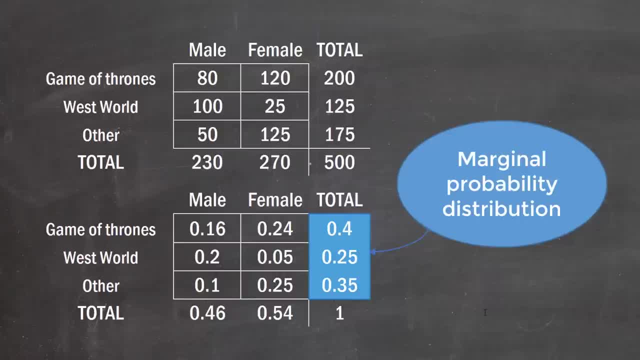 Now, of course, this actual column here is called the marginal probability distribution. So just like we had the joint probability distribution, this one I've highlighted here also sums to one. Now, the thing to appreciate is that this marginal probability distribution completely ignores gender. 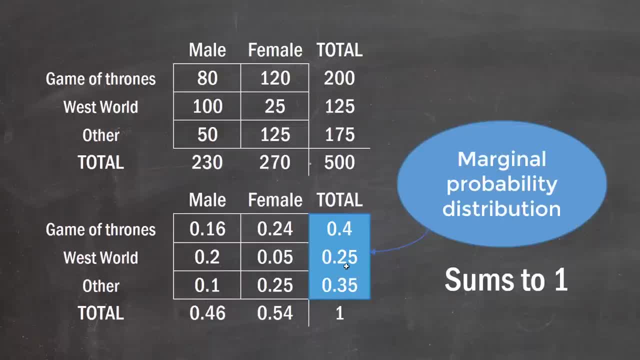 It's as if that variable doesn't exist here. but be aware also, there's another marginal probability distribution down here And in this case it would ignore the show of preference. But again, this is going to sum to one because there are 46% males in our sample. 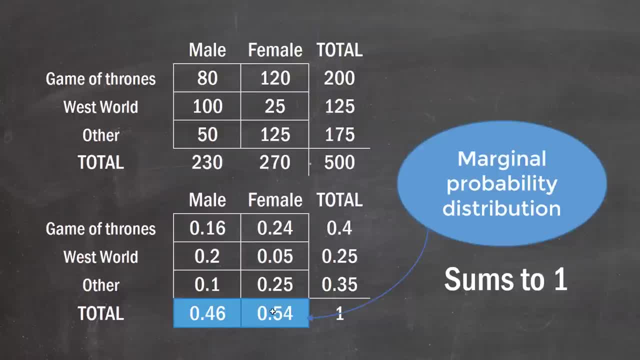 and 54% females in our sample, and we're gonna have to sum them up to get 100%. So our joint probability distribution adds up to one, but so does both of these marginal probability distributions Okay, so here's a couple of questions for you. 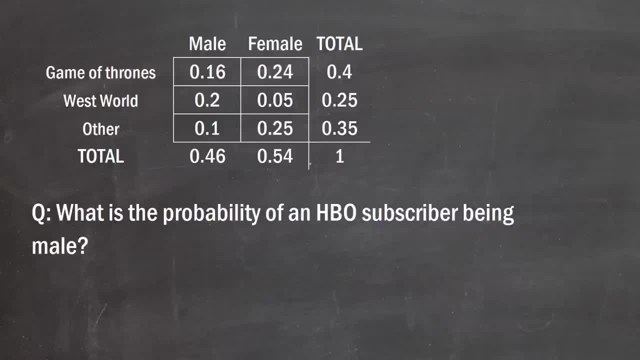 Just using what we've gleaned from the last minute or so, you should be able to answer some of these questions. What's the probability of an HBO subscriber being male? Now, I think I might've even said this before, but the probability of a subscriber being male? 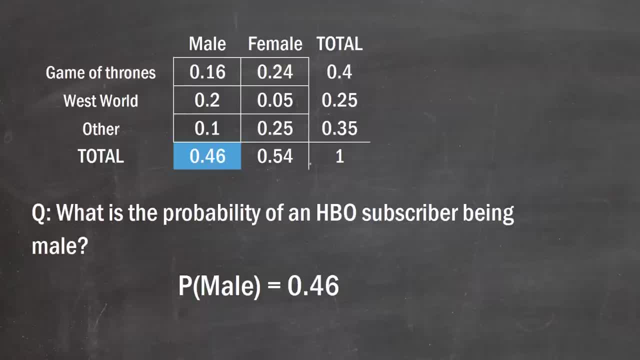 is purely that marginal probability of the male column, so 0.46.. Now just be aware of terminology. When we say probability, we're after a number that's between zero and one. Sometimes they'll ask about percentages and stuff, so you can turn that into a percent. 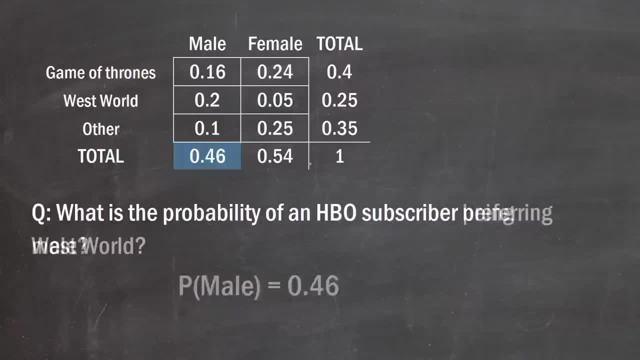 but if it just says probability, you can just leave it as 0.46.. Well, the next question: what's the probability of an HBO subscriber preferring Westworld? Pretty simple, it's just gonna be the 0.25.. So we can keep going. 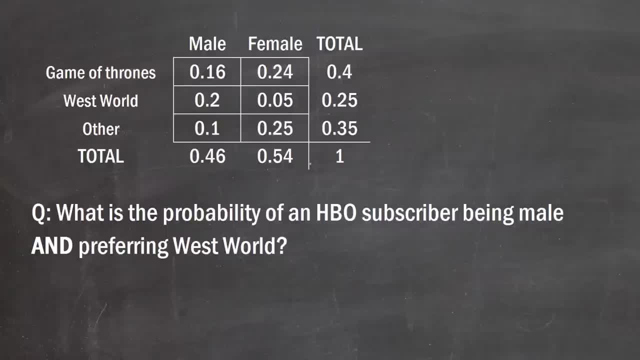 appreciating that those first two questions were asking for marginal or simple probabilities, This question asks: what's the probability of an HBO subscriber being male and preferring Westworld? So that's 0.2.. And again you've got that intersection symbol here. 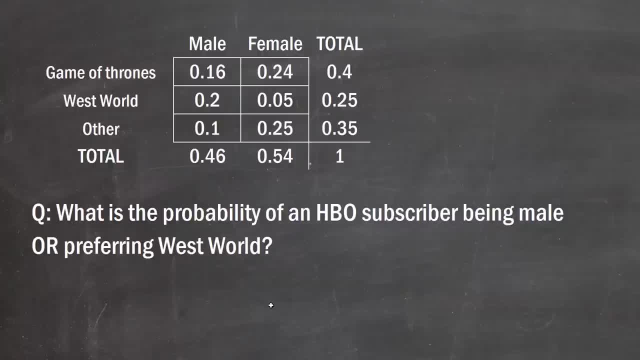 Now here's a slightly different one. It says: what's the probability of an HBO subscriber being male or preferring Westworld? So this is not an intersection, It's not a joint probability. It actually requires us to think just a little bit. 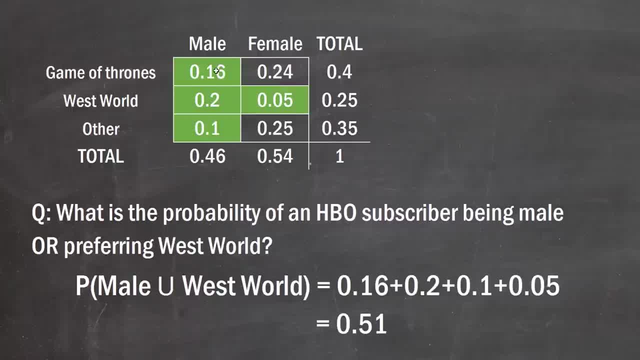 and appreciate that to find this we're gonna have to sum up all of the joint probabilities where these conditions met. So if the subscriber is male, we're in this column, so we can highlight these three cells green and we can also highlight the Westworld row green as well. 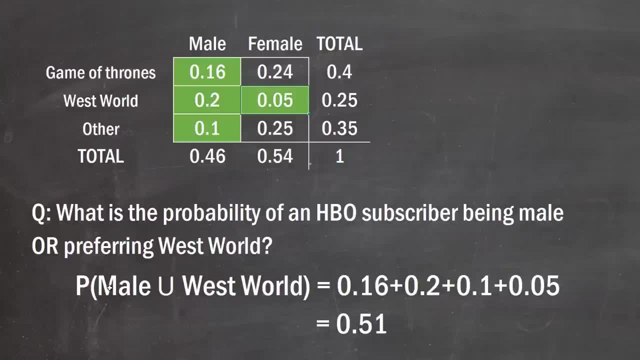 So in summing up those four cells, we're gonna be able to get this probability And you can see here I've just gone all of those numbers added together and I've got 0.51.. Now you might've noticed I used this upwards U here. 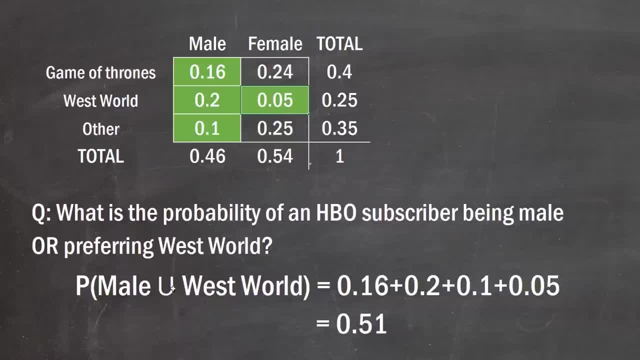 and this is the symbol that we call union. So this is the union of two events: of someone being male and the event Someone liking Westworld. Now, if you've watched a few of my other videos, you might know that I tend not to like formulas too much. 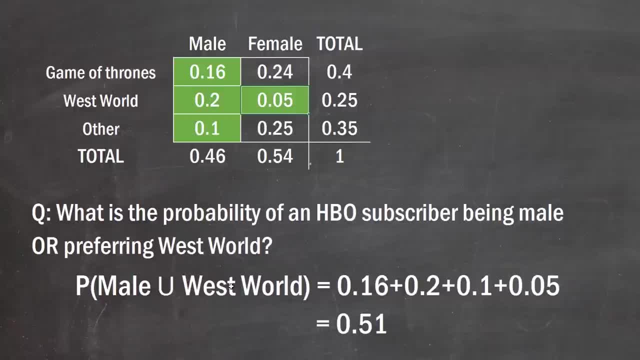 because formulas tend to stop us thinking And many of them have an intuitive basis to start with, And this is true of this formula here, which provides us a way of calculating the union between two events- So you might've seen this somewhere- where we say the union between events A and B. 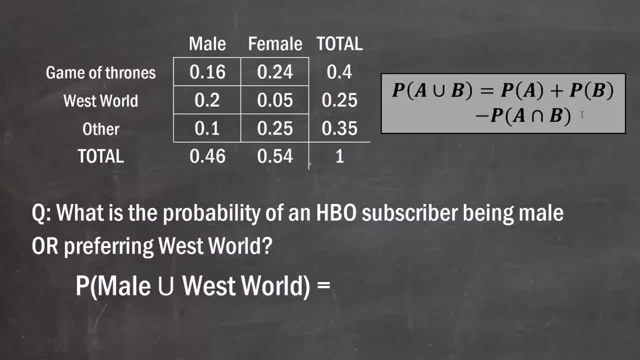 is the probability of A plus the probability of B minus the intersection. And again, you can calculate this one that way, if you'd like, which is to say that we add up the two marginal probabilities, the 0.25 and the 0.46,. 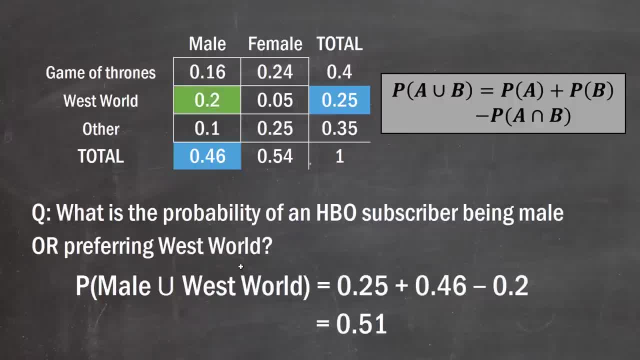 and then we subtract the joint probability at 0.2.. Now, why do we subtract the 0.2?? Well, if you think about each of these joint probabilities, this one here sums up the entire row for Westworld. This one here sums up the entire column for male. 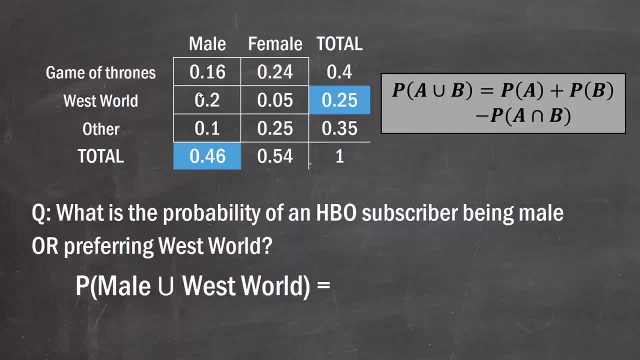 Thus we've actually added this cell twice the male Westworld joint probability. We've added that twice If we've just simply added these two blue cells together. So we have to subtract one of those away again to be left with 0.51,. 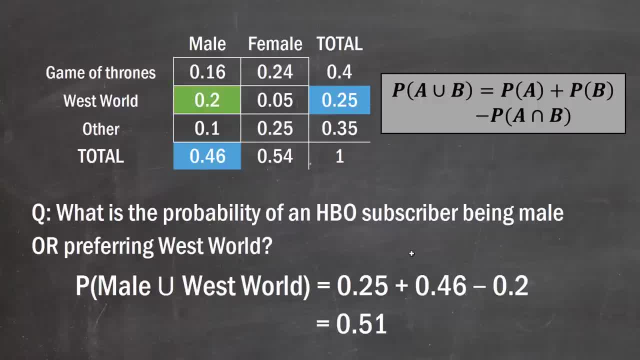 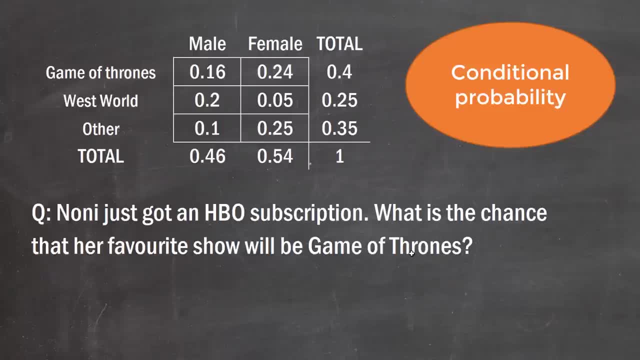 which is no surprise- the same answer we got using the other method. This brings us to the next and more tricky type of probability, which is called a conditional probability. So here I've given you a question again as an example: Noni just got an HBO subscription. 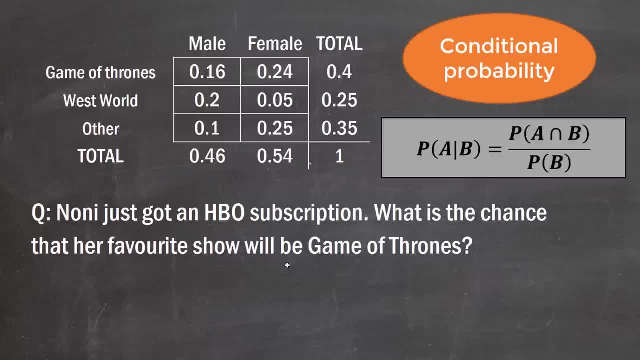 What's the chance that her favorite show will be Game of Thrones? Now again, you might've seen a formula that looks a little bit like this, where this says: the probability of event A given event B equals the intersection of the two events divided by the probability of the condition. 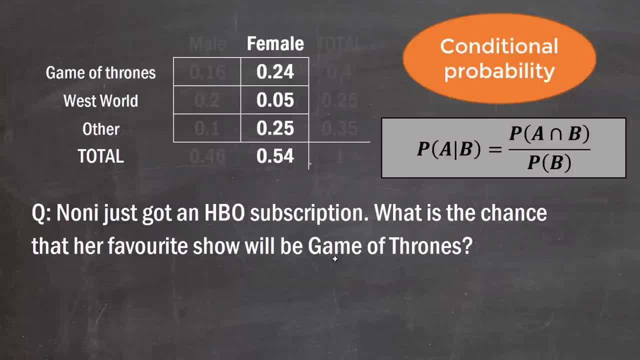 So in this case, what we do is we basically focus on the part of this distribution which is of interest And because Noni is female, we can ignore the rest of the table completely. We're only really considering this column here. We take the joint probability, which is 0.24,. 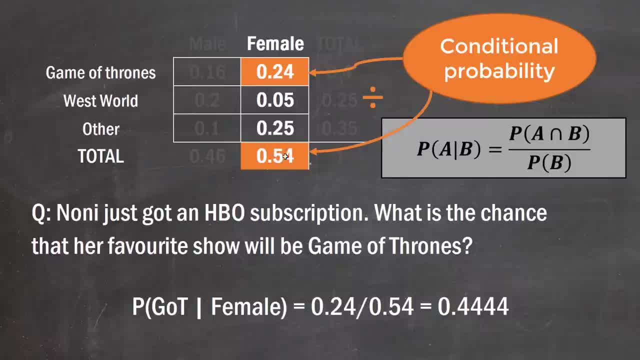 and we divide by the probability of the condition, which is 0.54.. Now the condition was that she was female. That was given in the question. So we can calculate this as 0.24 divided by 0.54,. 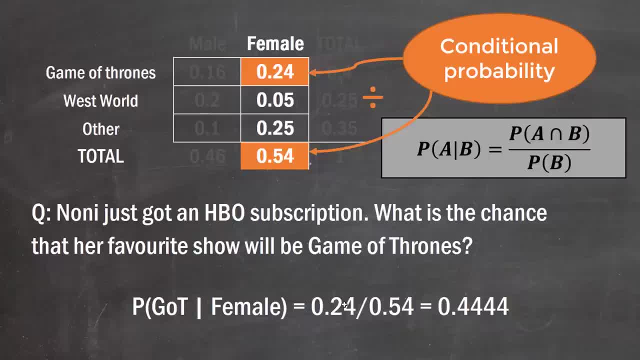 which is 0.44444, which is about four ninths, but that's okay, We can leave it as a four decimal place probability here. So what we can do now is create for ourselves a new column, which is the probability of preferring each of these shows. 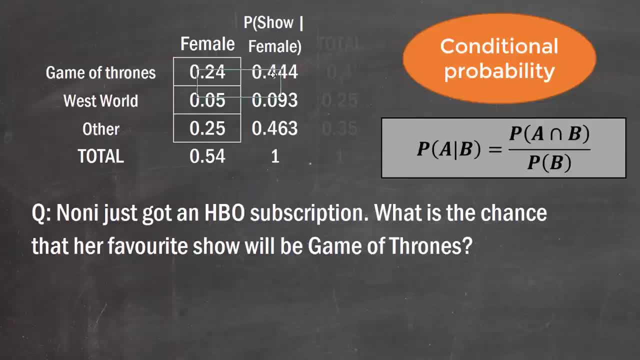 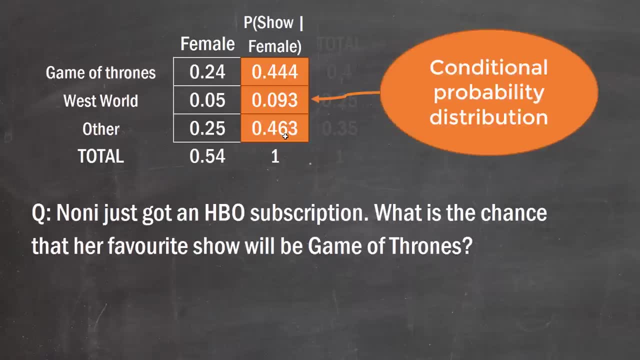 given someone is female. So we just got 0.44444 for Game of Thrones here. Now we can do the same for Westworld and other. We find here what's called the conditional probability distribution, So this is the probability distribution of preferring various shows, given someone is female. 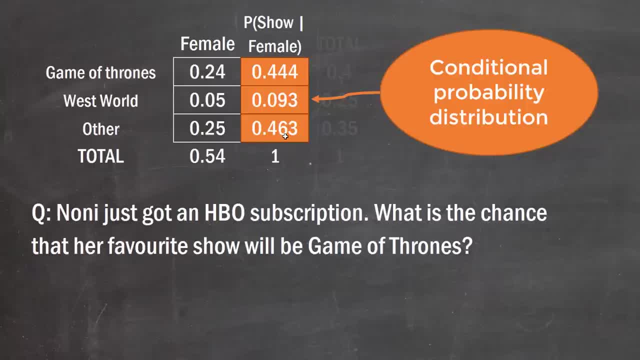 And again, because it's a complete probability distribution, it's going to add up to one, And indeed this does So. what we can do now is we can compare this conditional probability distribution to the marginal probability distribution. That's this one here, the original total distribution. 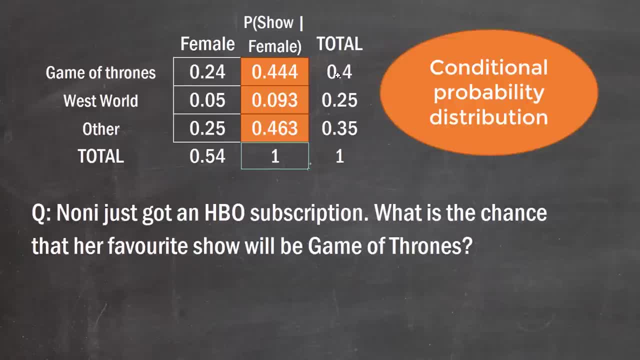 And we can see that if we don't take sex into account, 40% of people like Game of Thrones, 25% like Westworld, 35% like other shows. But when we take gender into account, these change a little bit. 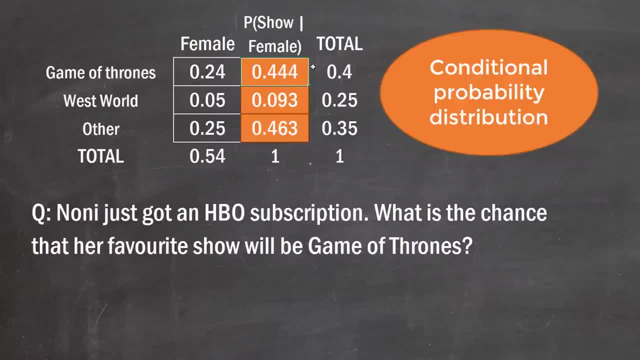 So for females, you can see that they're more likely to like Game of Thrones than the general population. they're less likely to like Westworld than the general population And they're a little bit more likely to like other shows than the general population as well. 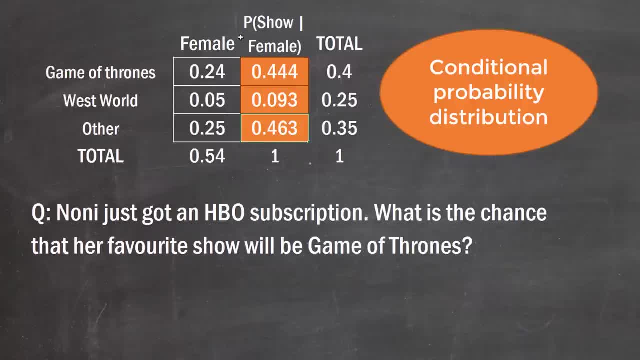 And we can actually use this to assess whether the two variables, gender and show choice, are independent. But before we do just appreciate that, we can also go the other way with our conditions. So for example, if I asked you, given that a subscriber's favorite show is Westworld, 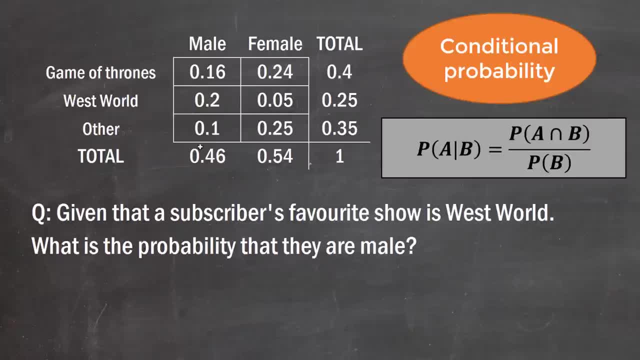 what's the probability that they are male In this case, the condition is that? well, the condition is that they like Westworld, So our condition is actually an entire row, So, much like last time, we can block out the rest of the table that doesn't coincide with Westworld. 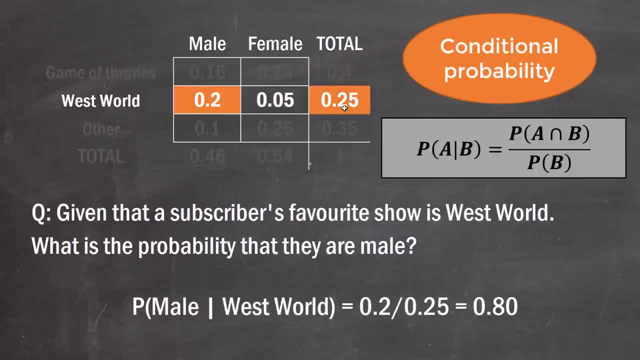 And we can just focus on this row. And the probability of being male is that 0.2, which is the joint probability divided by the probability of the condition 0.25.. So if you do that, you get 0.8,. 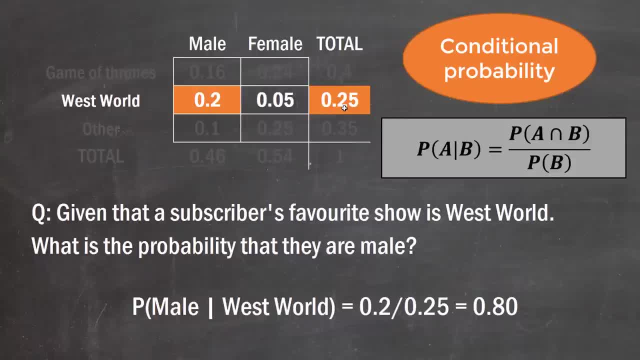 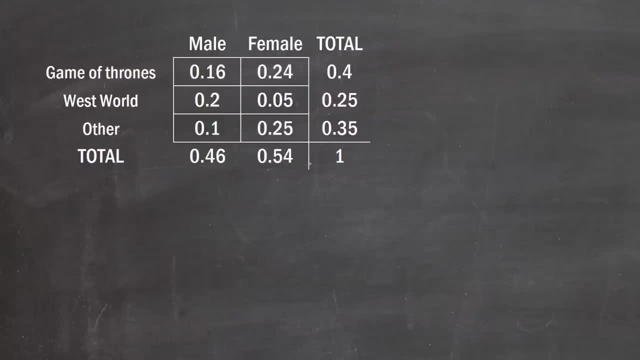 and that's the probability of being male, if you prefer Westworld. In other words, 80% of people that watch Westworld are males. So this leads us to the topic of independence between the variables. Now, we've already touched on it, just briefly. 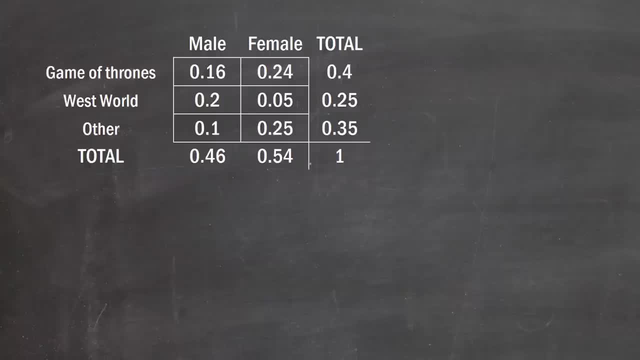 to show that females have a little bit of a different preference of their HBO shows to the general population. But the strict definition of independence actually has two different approaches, The first of which says that if the two variables are independent, then the probability of age 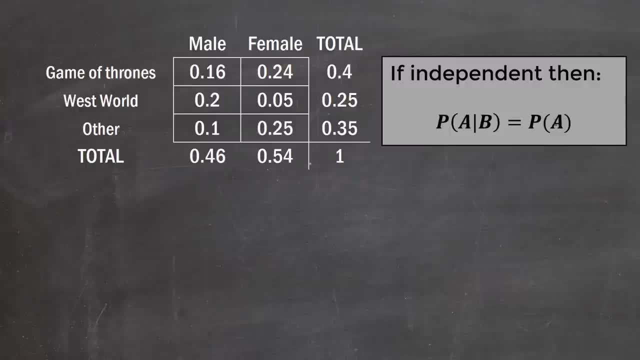 given B is just equal to the probability of A. Another way to think of this is that imposing the condition B doesn't actually affect the probability of A at all. So in our case we found the probability of liking Westworld if you're female is 0.093. 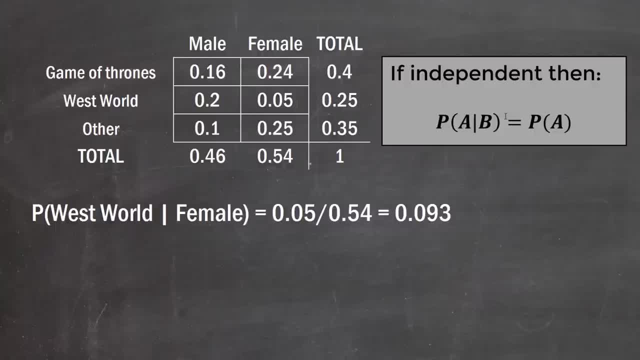 We found that from our conditional probability distribution earlier. But the probability of just preferring Westworld straight up is 0.25.. It's in that final, It's in that marginal value here. It's in that marginal value here. So if these two variables 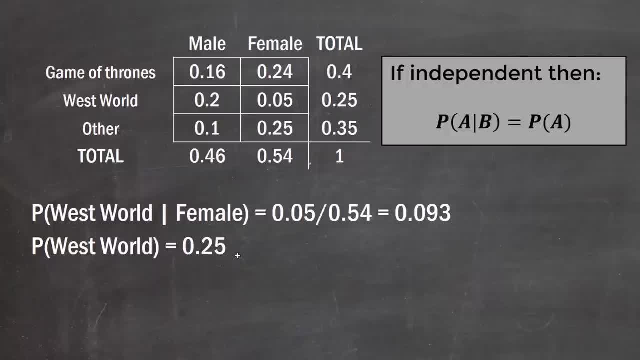 gender and choice of HBO shows were independent, these two values should be equal. Therefore, the variables are not independent, as 0.093 does not equal 0.25.. So clearly, gender does influence the HBO show that they prefer. Now, it's probably worth mentioning that. 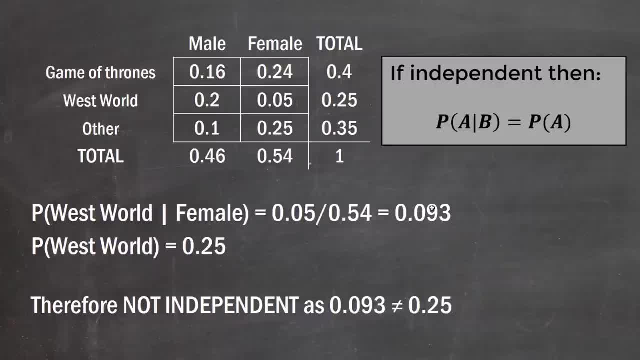 because this is a sample. you would never expect for these values to be exactly equal, Because we know in a sample there's going to be some random variation And even if the variables were completely independent, these two probabilities wouldn't be perfectly equal. 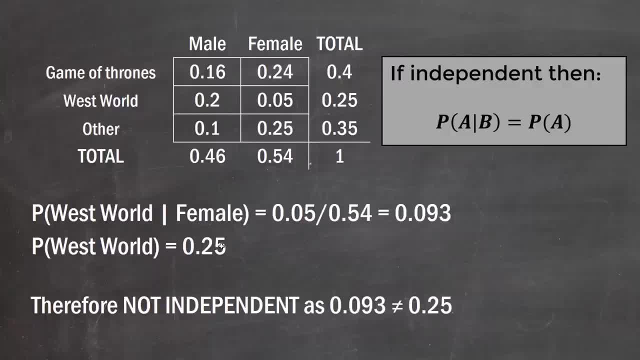 But in this case, I think it's quite clear that they're very different probabilities- One's 25% and one's 9%- So I think we're quite safe to say these variables are not independent. Now, as I said, there were two approaches. 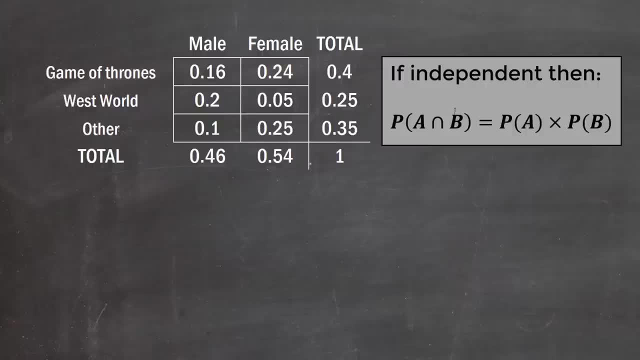 for assessing independence, And this one, I think, is a little bit different. This one says: the probability of A union B is equal to the two marginal probabilities multiplied together. Now I've got a feeling you might understand this equation intuitively, So if I can take you away from this example, 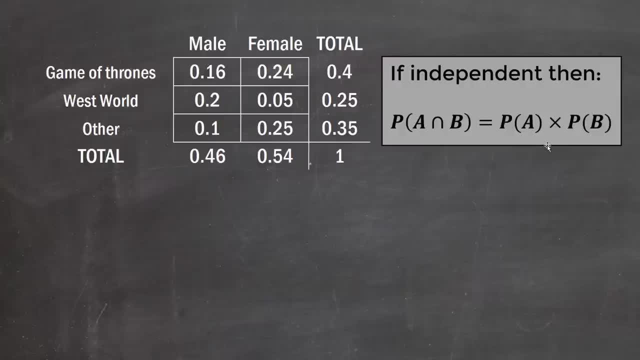 just for a second. say, I flipped a coin in one hand and I rolled a dice in the other hand and I said I'm going to give you a hundred bucks if I roll a six and I flip a head. If both of those events occur, I'll give you a hundred bucks. 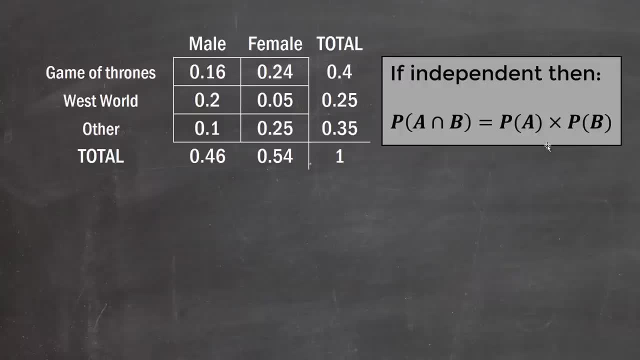 And I asked you what is the probability of me giving you a hundred bucks? You'd probably say, well, that's one in 12, right? Because you've got half a chance of getting a head and a sixth of a chance of rolling a six. 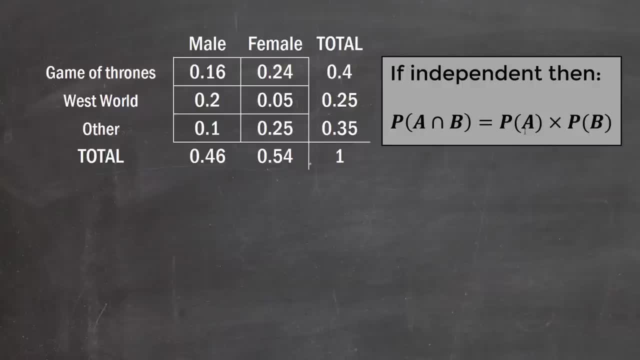 So you multiply them together, You're going to do the probability of A getting a head times the probability of B and you're going to get that joint probability. But the only reason you can do that is because rolling a dice and flipping a coin. 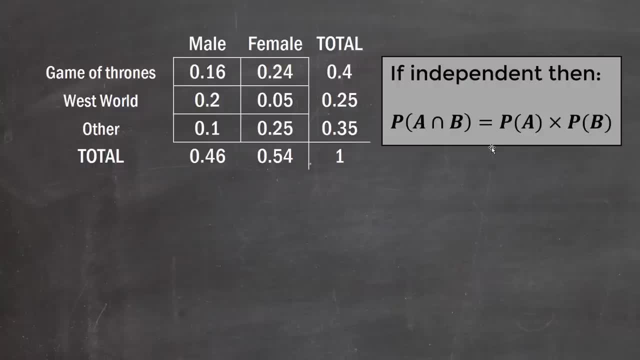 are completely independent variables. It's not as if rolling a six influences the chance of getting a head right. So, as I said, you can kind of intuitively understand this formula. But what that implies for our distribution here is that if we were to look at the intersection, 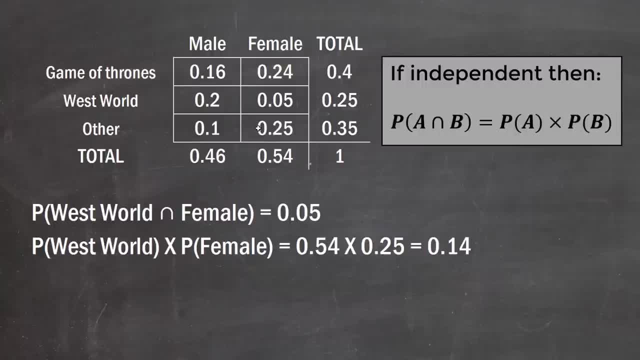 between Westworld and female, we get 0.05.. And if you multiply the two marginal values together, the 0.54 and the 0.25, you get 0.14.. So again, these two values are not the same. 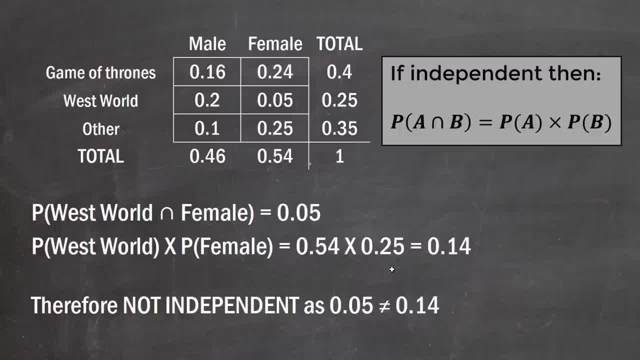 So we can say they're not independent variables, Which is no surprise, because we just showed this using the other approach. So either of these approaches would be fine to show that people's preference of HBO shows does depend on their gender. All right, so that's a wrap.